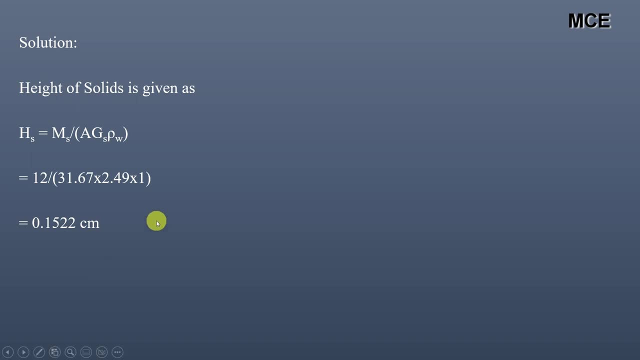 into which is equal to 0.1522 cm or 1.522 mm After the value of height of solids. Now we will draw the compression curve. To draw the compressor curve we need to find the change in volume. higher pressure, iteration, presure intervals. And for that we will use excel. So let's moved to Excel. let us move to excel. The key point we will use is in the data data. Now we will also see the Laplace rotation percentage of solids. Let us move to excel. So let us move to excel, and we will take a look at the expression equation. 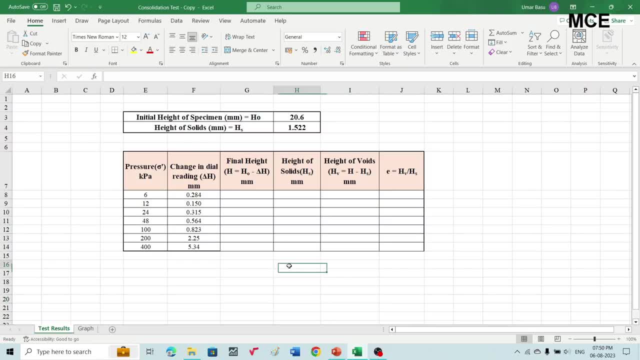 So let us move to excel. to do the required calculations In excel, you will first draw a table having six columns in which the first column will be the pressure values and second column will be the change in dial gauge reading in mm. Both of these are already given in the question. 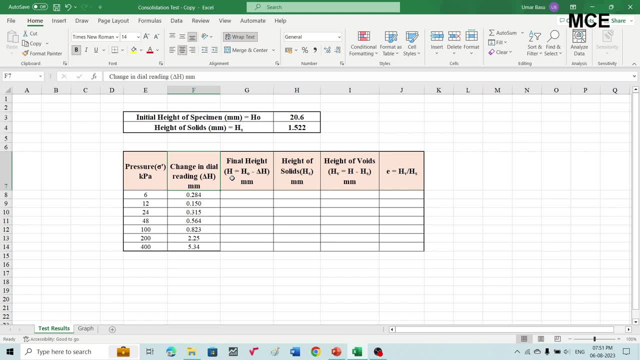 Third column is the final height, which is equal to initial height minus change in dial gauge reading. So for pressure of 6 kPa, final height will be the initial height of the specimen, which is 20.6, minus change in dial gauge reading, which is 0.284.. 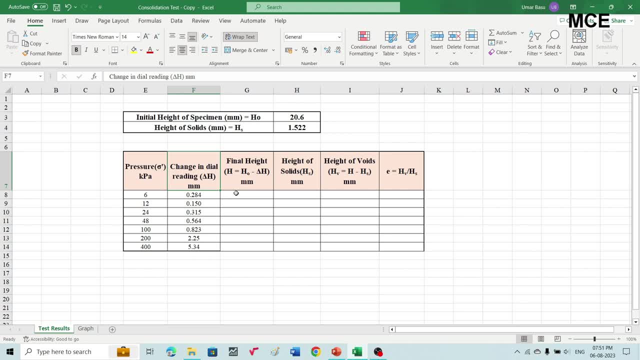 So you will select the first row of final height at pressure of 6 kPa and then write equal. then you will select the initial height of the specimen, which is 20.6, or you can directly write 20.6. then after that you will write minus sign and then you will select the change. 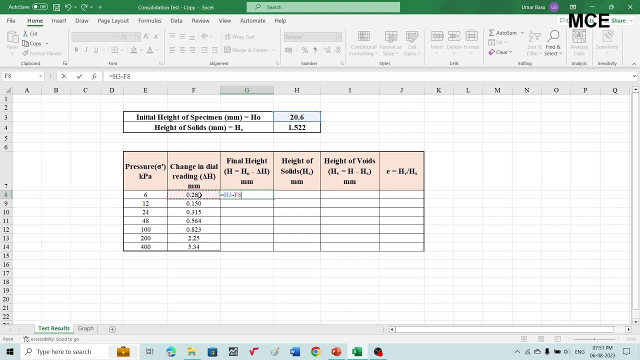 in dial gauge reading At pressure of 6 kPa, which is 0.284, and then press enter and you will get the final height of the specimen at pressure of 6 kPa. For the next pressure, which is 12 kPa, initial height will be the final height at 6 kPa, which. 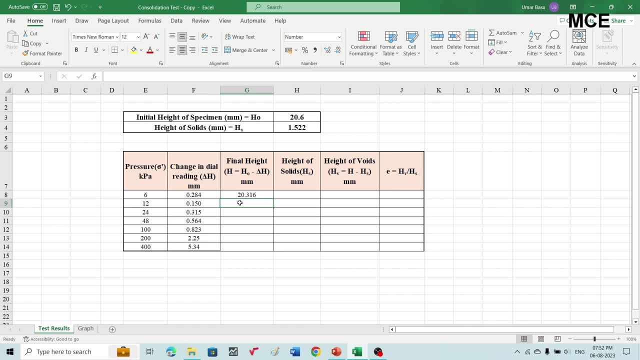 is 20.316. so you will write select this row and then write equal sign, and then you will select this 20.316 value and then write minus. Then you will write minus. Then you will select the change in dial gauge reading at pressure of 12 kPa, which is 0.150. 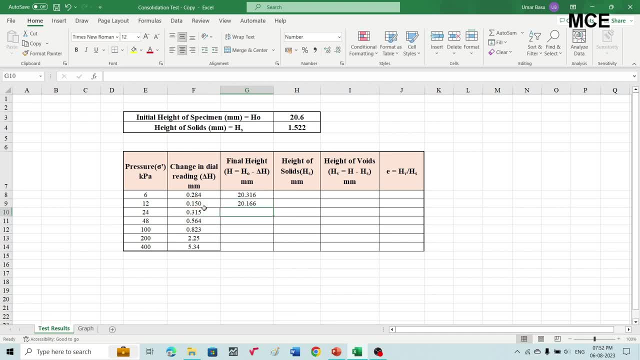 and press enter and you will get the final height at pressure of 12 kPa. To get the final height at rest of the pressure values, you will select final height at 12 kPa and then you will drag it till the last row and XR will automatically calculate the values. 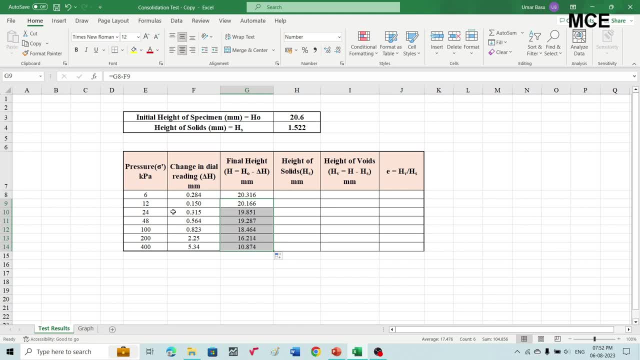 for value of final height. for rest of the pressure values, Height of solids calculated and this is equal to 1.522. so you will write equal sign and then write 1.522. this is the height of solids, since height of solids is same for all the pressure values. so you will select. 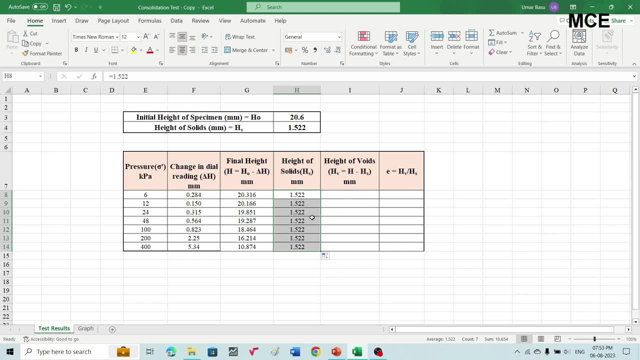 the first row and then drag it till the last row and you will get the values for different pressures. now, height of voids, this is equal to the final height minus the height of solids. so for pressure of 6 kilo pascal, you will select the first row and then at equal sign, then you will select the. 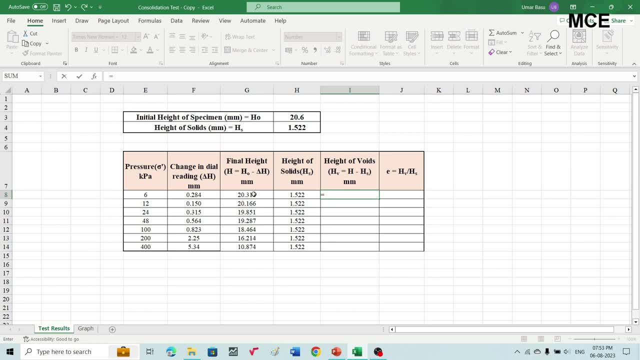 final height at pressure of 6 kilo pascal, which is 20.316. then write minus sign and subtract it the height of solids, which is 1.522, and press enter and you will get the height of voids at pressure of 6 kilo pascal. to get the value of height of voids for rest of the pressure select: 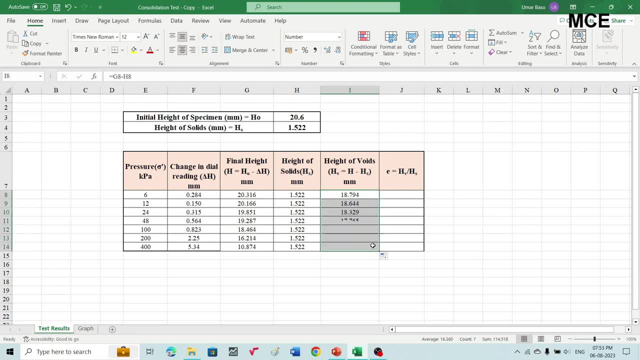 the first row and then drag it till the last row and you will get the height of voids. for rest of the pressure values void ratio, this is equal to the height of voids divided by height of solids. so for the first row you will write equal sign. then select height of voids at pressure of 6 kilo pascal. divide it by. 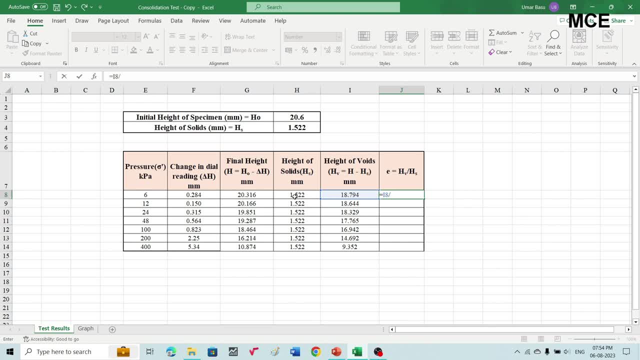 height of solids, which is 1.522, and then press enter and you will get the void ratio at pressure of 6 kilo pascal. for rest of the pressure values: value: select the first row and then drag it till the last row and you will get the 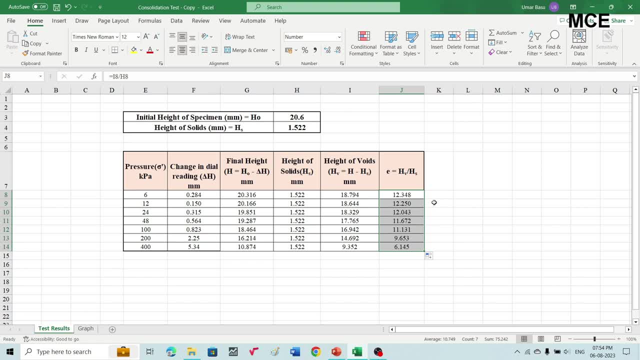 void ratio at different pressure values. After getting the value of void ratio at different pressure values, we will plot a graph between the pressure value and the void ratio values with pressure values on log scale and void ratio value on natural scale to get the compression curve. 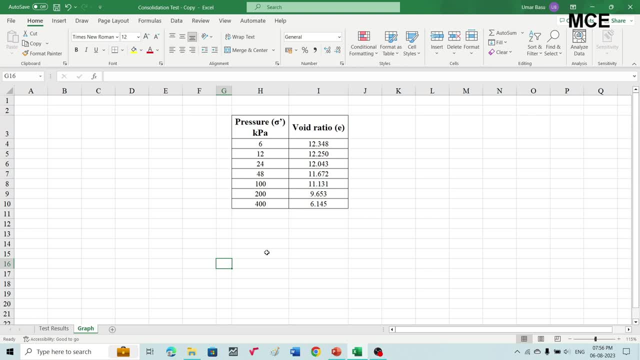 Now to draw the compression curve, you have to make a table in excel having two columns. The first column will be the pressure values and second column will be the void ratio values. Then, to draw the compression curve, you will select the values and then you will click. 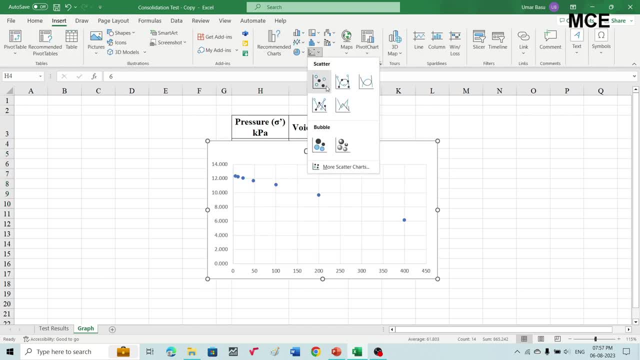 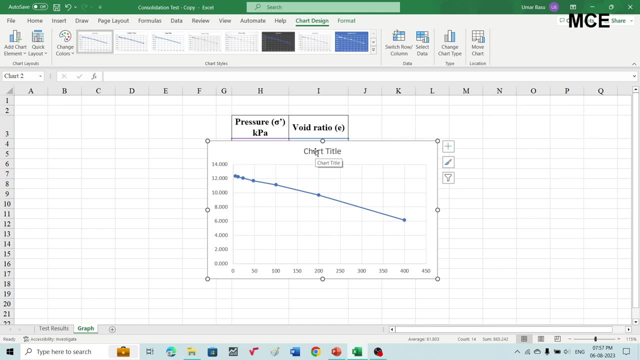 on the insert. Then you will click on the charts and you will select this, that is, scatter with straight lines and markers, and this will give you a graph between the pressure values and the void ratio values. First you will delete this chart title and then click on this plus sign. 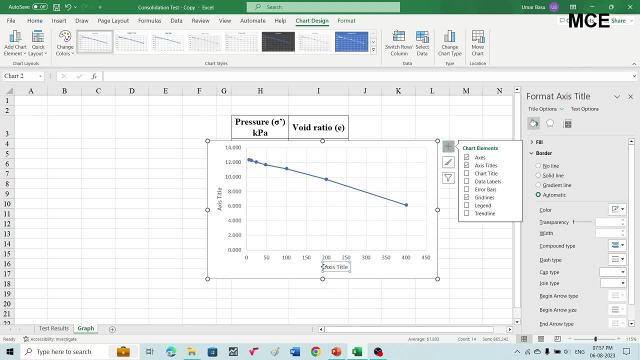 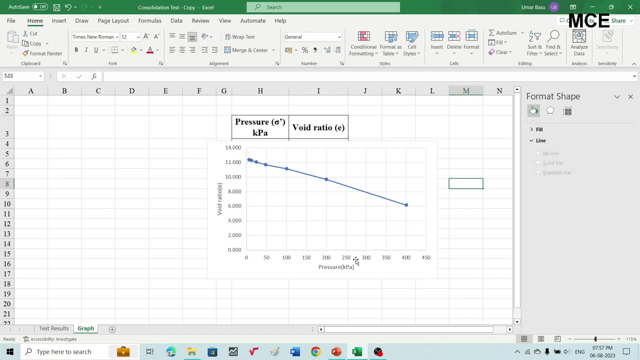 Then you will add the axes title. For horizontal axes you will write the pressure in low pascal, and for the vertical axes you will write void ratio, Since for compression curve pressure values need to be on the logarithmic scale. so you 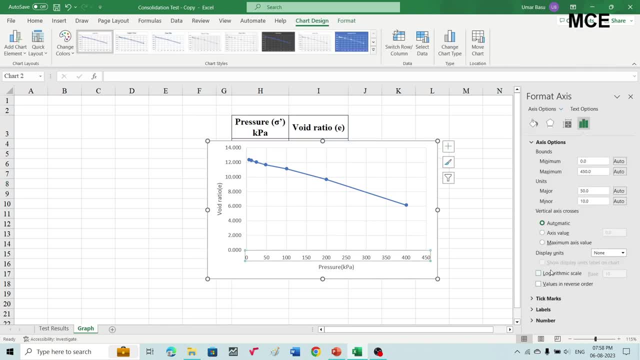 will select the horizontal axes and you will change it to the logarithmic scale. After that, you will also make this tick marks visible for major type, as cross, and minor type, as inside, And also you will You will change the color of this axis to make these tick marks more visible. 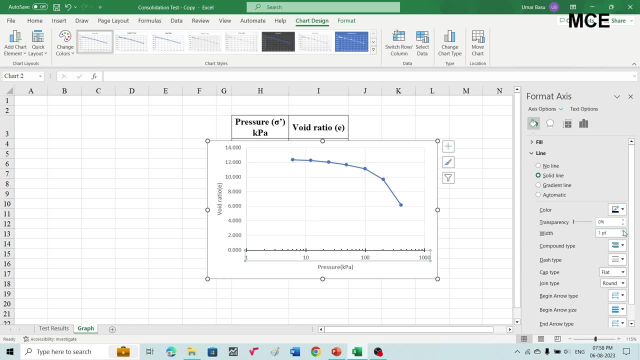 So change it from gray to black and increase the weight to one point. You can now see the values. similarly for the vertical axes. You will select the vertical axes, change its color from gray to black and increase the width to one point. And in the axes option, 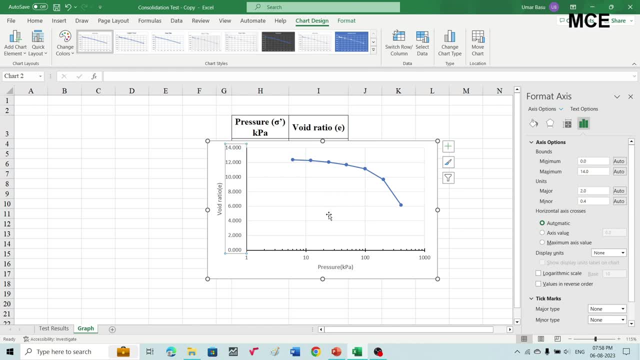 You will take the. We can see that The no value of void ratio is less than six, So we'll write the minimum as five and maximum will be 13.. And also for units, you will take the minor one as zero point five. 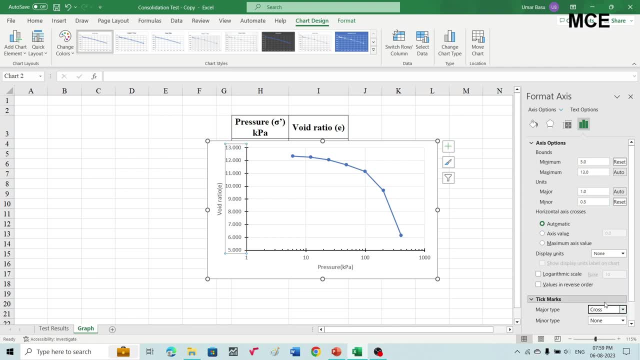 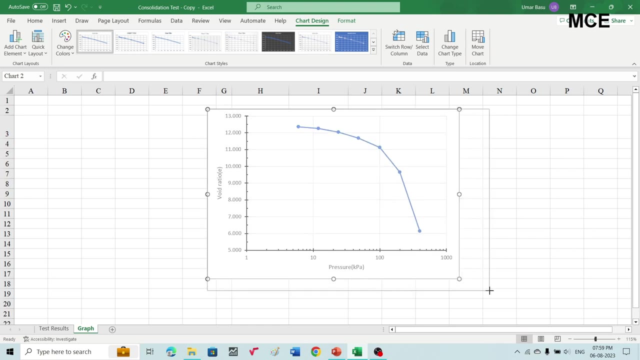 And you will again make the tick marks visible for major type as cross, and minor type, as inside. You can Now see that This is our compression curve. You can increase the size of the compression curve To see the graph more clearly. Okay, 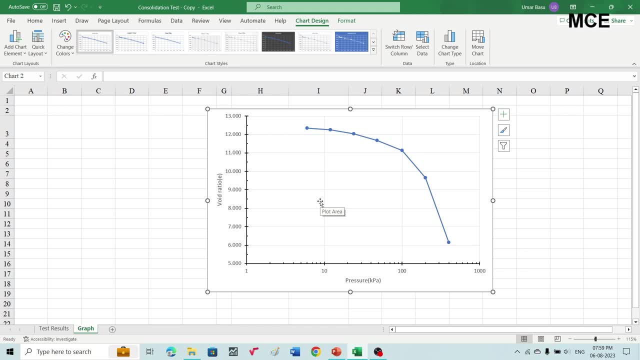 So this is our guide: compression curve. to get the value of pre consolidation pressure From this compression curve, we have to select a point on this girl that will have the having the Maximum Curvature. So the point having the maximum curvature On this point. 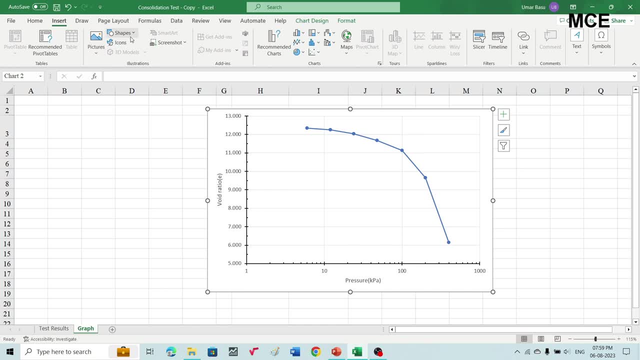 That is this point. This point is having the maximum curvature. You will first draw a horizontal line. So draw a horizontal line on this point: Having the maximum curvature or minimum radius of curvature. After drawing the horizontal line also, you will draw a tangent at this point. 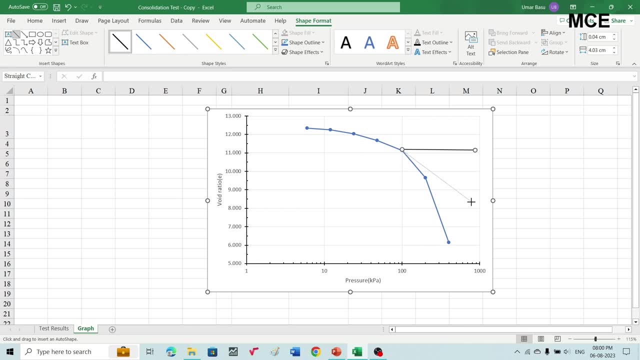 So draw a tangent at this point. Then you will Bissect the angle between the horizontal and the tangent. So bissect the angle. Okay, After bisecting the angle, You will extend the straight line portion of this graph, Which is: 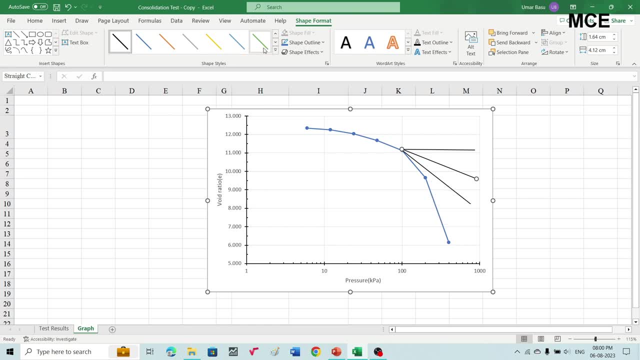 this graph. this is the straight line portion of the graph, so we will extend it. so, extend this straight line portion of the graph and we can see that this will touch this bisector at some point. okay, the point where it touches this bisector. from this point you will draw a vertical line. 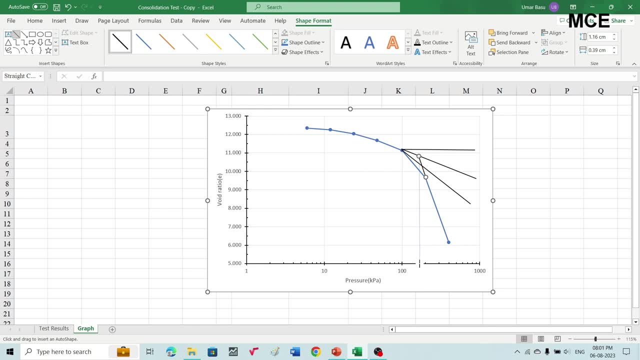 so draw a vertical line from this point. the point where this vertical line touches the horizontal axis gives you the value of pre consolidation pressure. so we can see that first value. this value is hundred kilopascal and the second value is 200 kilopascal. this point falls between: 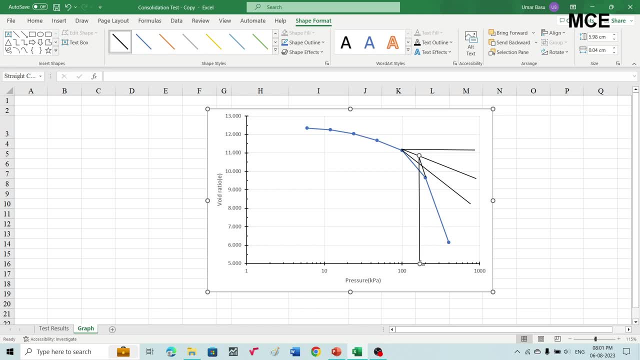 100 and 150 is the pre consolidation value in this graph. so now in this representation, and 200 kilo pascal, and it's close to 200 kilo pascal, so it's roughly equal to 185 kilo pascal. so you can see that the value of pre-consolidation pressure for this soil is 185 kilo pascal. 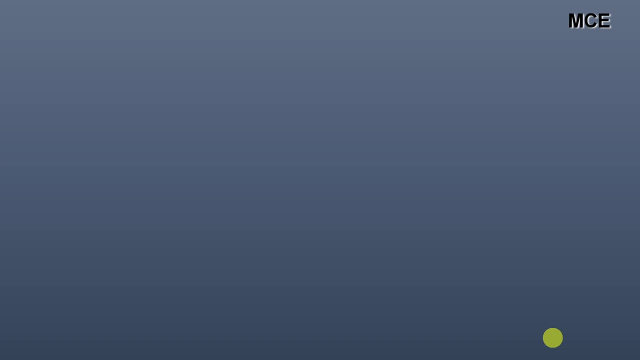 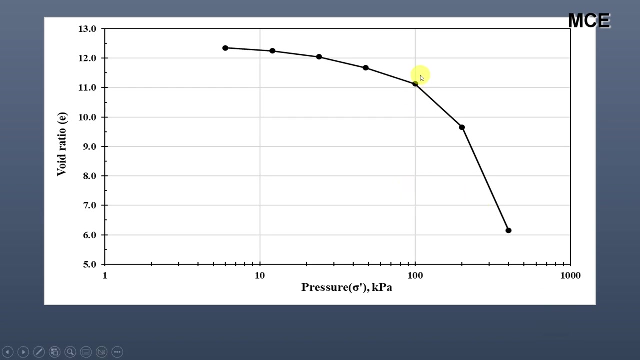 if i summarize the concepts of finding the pre-consolidation pressure. first you will select the point having the maximum curvature or minimum radius of curvature. from this point you will draw horizontal line. also, you will draw a tangent at this point. then you will bisect the angle between.